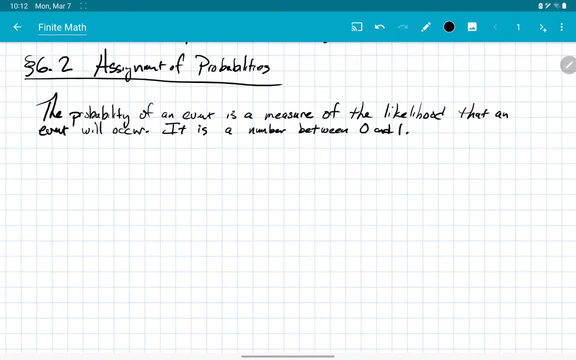 a probability to a percent, but it's a number between zero and one. And also notice that we talk about the likelihood of an event occurring, not an outcome. So we can take more a few outcomes and put them together in an event and then measure them. 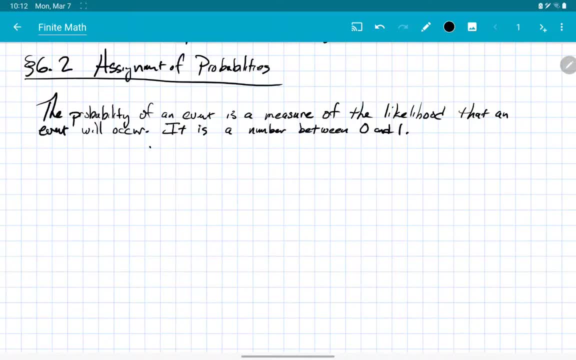 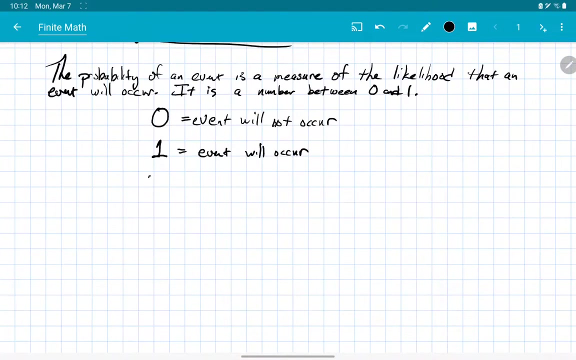 Okay, so zero. a probability of zero means event will not occur, A probability of one means the event will occur, And a probability of 0.5 means the event will occur half the time. So you're probably used to thinking about percentages, right, But you just slide the. 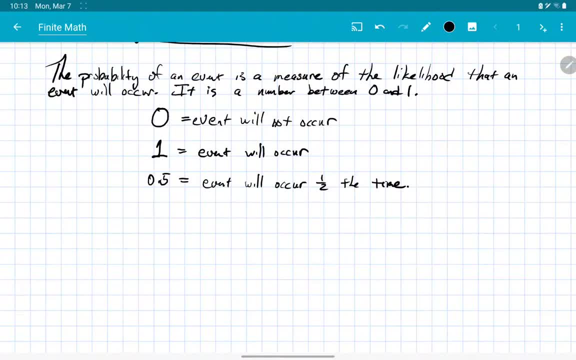 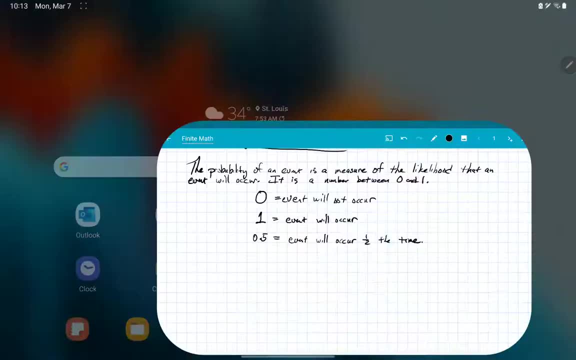 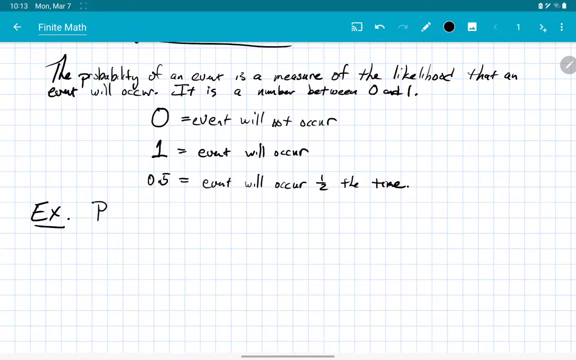 decimal point over too. That's the only difference here. Okay. so example Example: The probability it will rain tomorrow. We could look at the probability it will rain tomorrow And we could say that could be 0.3.. Okay, three times out of ten it will rain tomorrow. That necessarily means then the 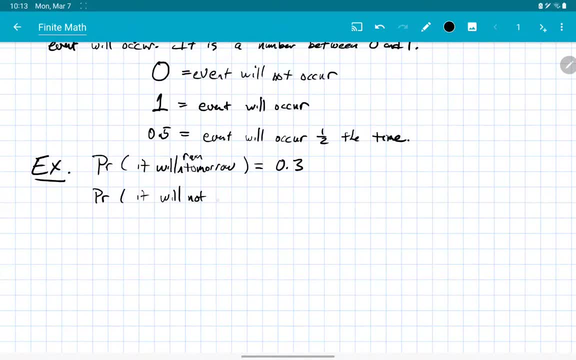 probability it will not rain tomorrow. Okay, it would be 0.7.. Because it will either rain or not rain. Those are the only two possible outcomes or options. So it will rain or it won't rain. So together that must equal certainty. 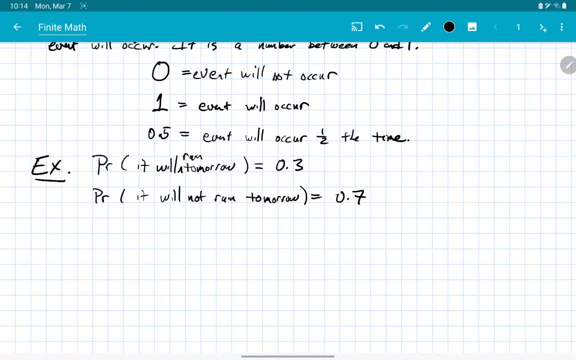 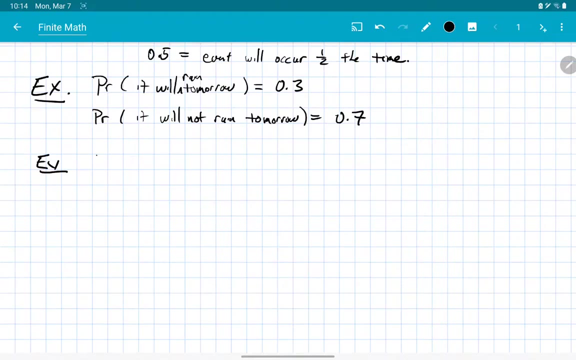 I can be certain, with probability of one, that it will rain tomorrow or it will not rain tomorrow. Those are mutually exclusive and they exhaust all possibilities, so the sum is one there. Now let's look at another example. Let's toss a coin two times. 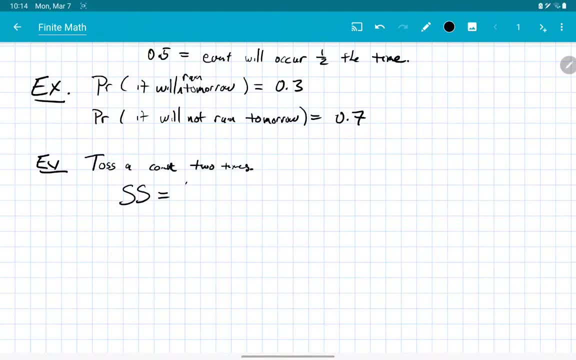 The sample space I'm going to abbreviate that SS unwisely looks like this: Heads, heads, Heads, tails, Tails, heads, Heads, tails, tails. Those are all the possible outcomes. That's the entire sample space. 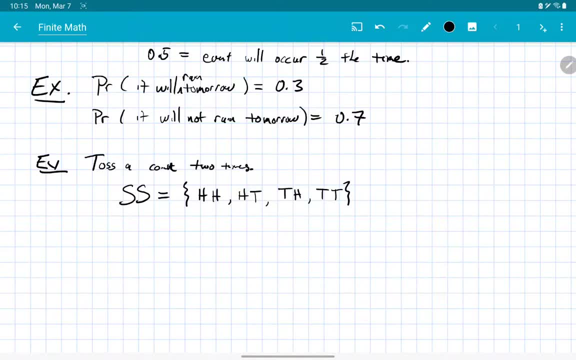 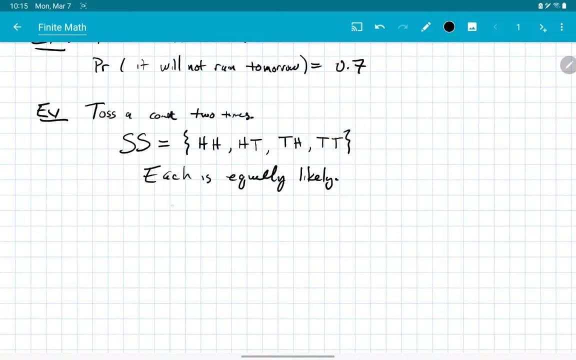 of what can occur for tossing a coin two times, And each of these is, of course, equally likely. So that means the probability of getting heads heads- is equal to exactly a quarter. A quarter of the time you should get heads twice in a row. 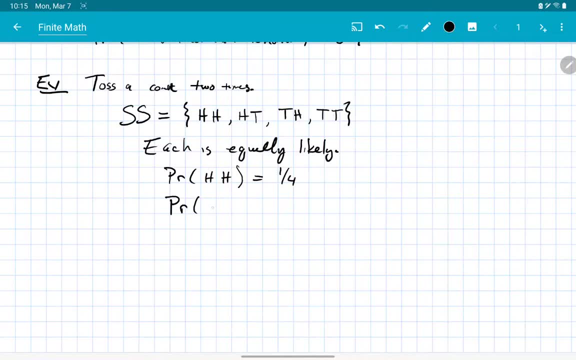 We could also look at a more complicated event, like the probability that we have at least one head. That would be okay. that one works, that one works, that one works. So it would be probability three-fourths Okay. if we put these in decimal, this would be 0.25. 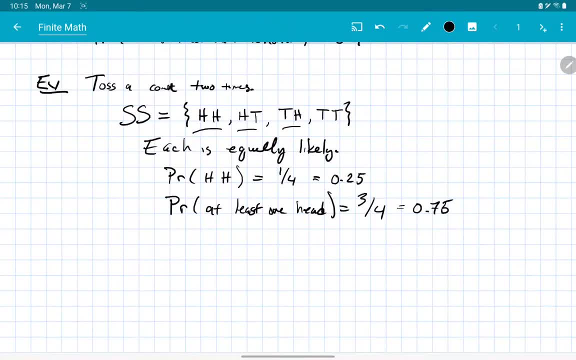 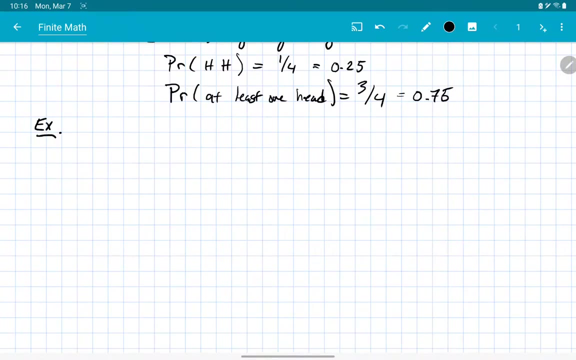 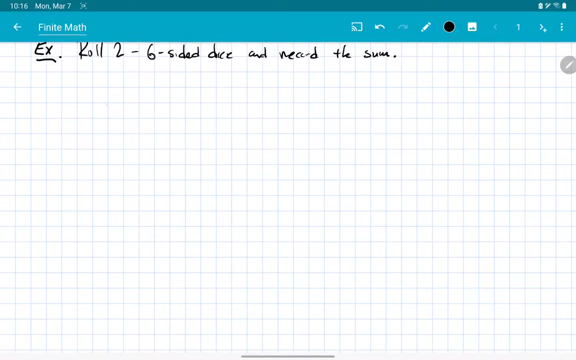 and this, of course, would be 0.75.. So that's another situation where we can easily assign the probabilities to what's going on. Now let's look at another example. Let's roll two six-sided dice and record the sum. So we'll make a table for this. 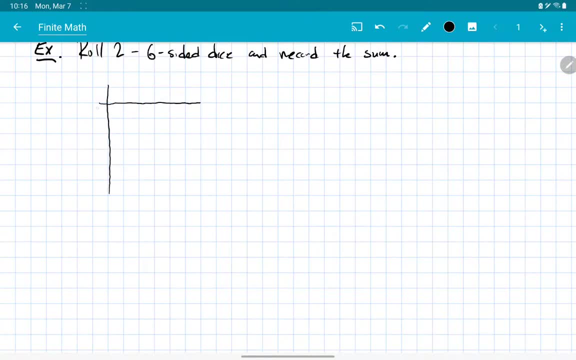 This is die one, die two. We can get one, two, three, four, five or six from die one. We can get one, two, three, four, five, six, possibly for die two. Those are our possibilities, right. 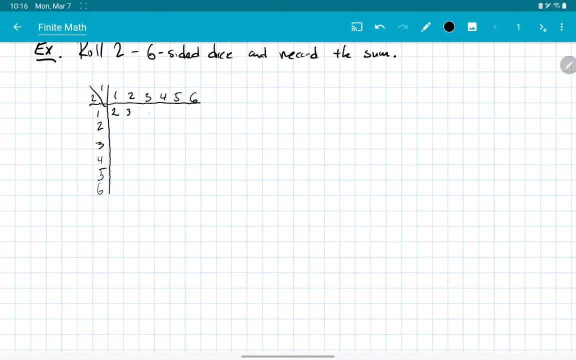 And now we record the sum of these numbers in the table. So two, three, four, five, six, seven, Three, four, five, six, seven, eight. So we can get one, two, three, four, five, six, seven. 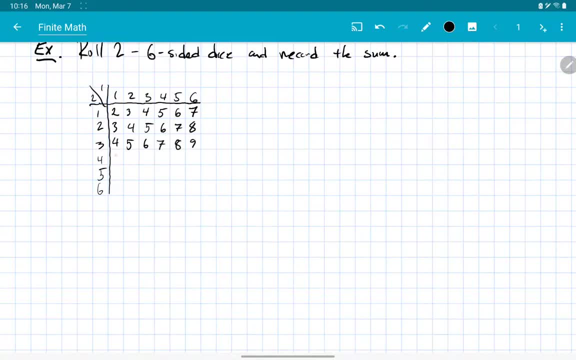 Four, five, six, seven, eight, nine, Five, six, seven, eight, nine, ten, Six, seven, eight nine, ten, eleven, Seven, eight, nine, ten, eleven, twelve. Okay, so there's all the possibilities. 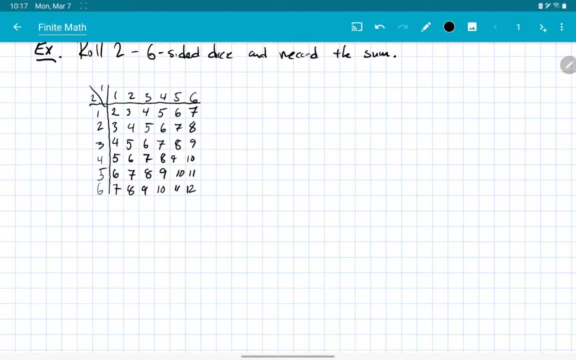 And now we can say: what is the probability of a sum of seven? Well, we look at this table, We note the sevens occur along this diagonal, here, And there are six of them, And there are a total of 36 total sum outcomes. 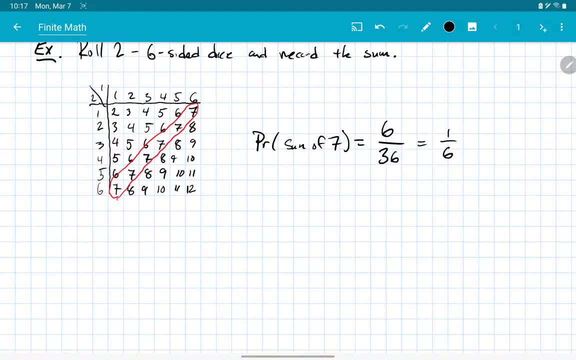 that we see in this table. So this would be six over 36, or one-sixth of the time. Is that about 17%, I think? I think it's .16 repeating. So one-sixth of the time you will get a seven. 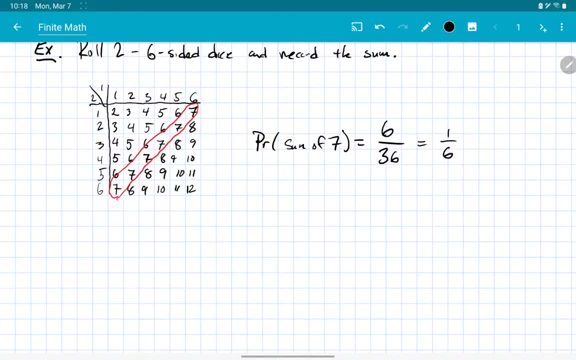 when you roll two dice, And then we could say: what's the probability of a sum of at least eight? Well then we circle. Okay, what is the probability At least eight is this portion, And I count how many things are there. 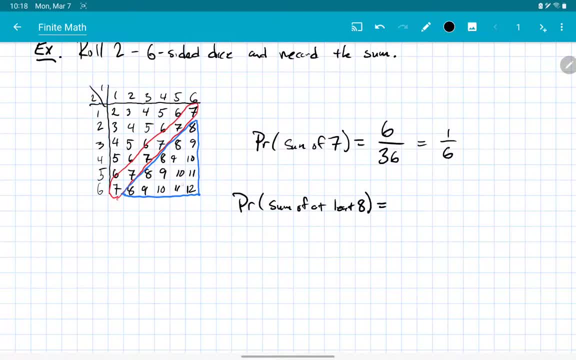 One, two, three, four, five, six, seven, eight, nine, ten, eleven, twelve, thirteen, fourteen, fifteen. This would be 15 over 36.. Okay, this is reducible, I believe, to five-twelfths. 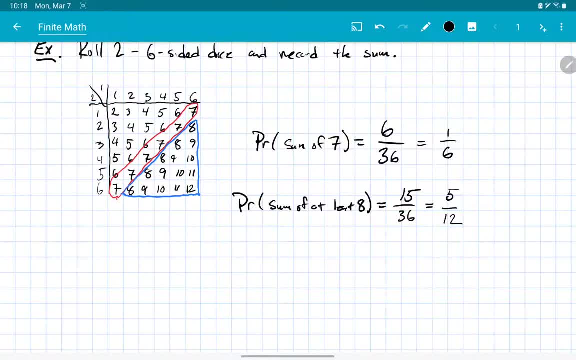 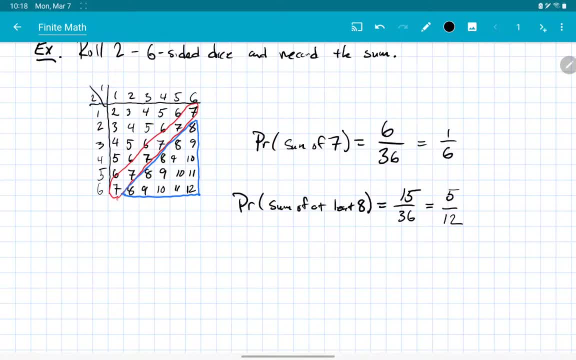 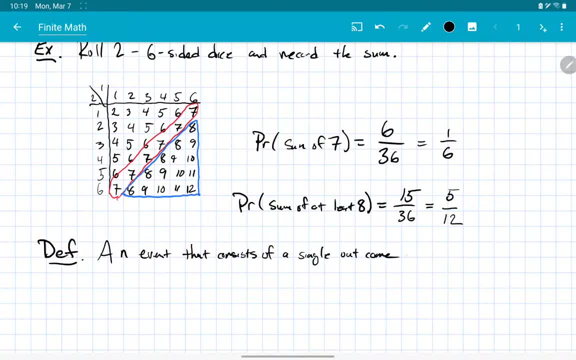 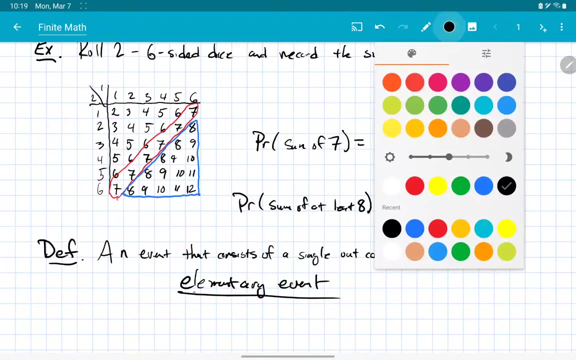 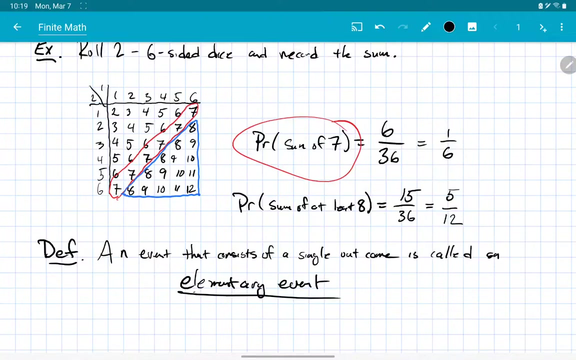 single outcome is called an elementary event. an elementary event. an example of an elementary event is this one: right here, since we're only right, the only outcome of recording is the sum of the dice. we're not. we're not thinking of different ways to get a seven, we're only recording the sum of the dice. 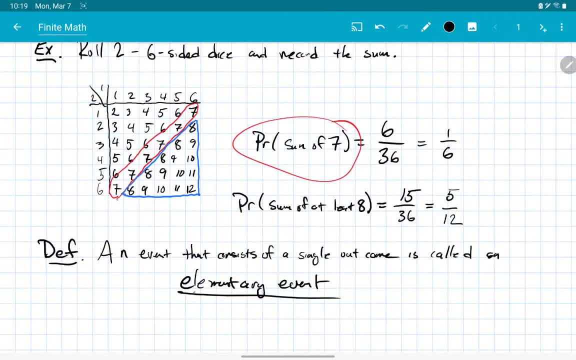 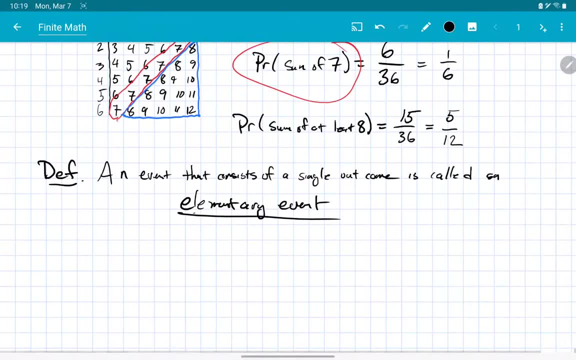 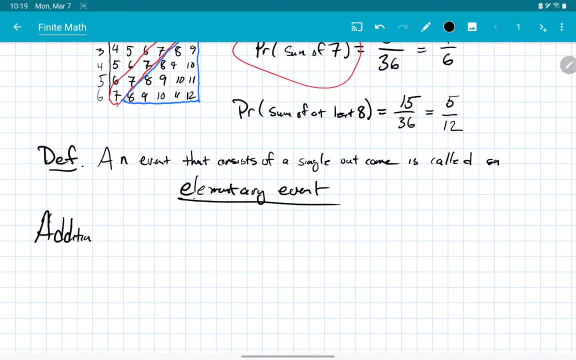 as the outcome, then a sum of seven is an elementary event. if we're only recording the sums, okay. so here is what they call the addition principle. so if an event e equals, say outcomes s, t, u, z and s? t? u, all the way to z, are single outcomes. 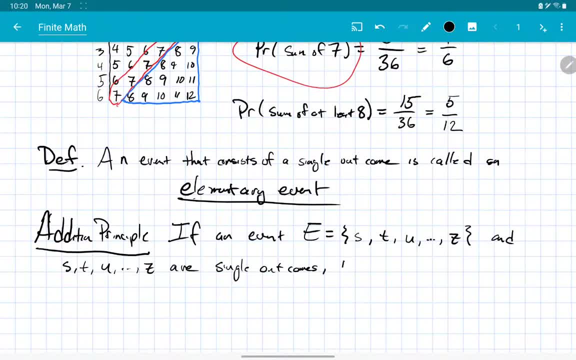 then the probability of the event e is the sum of the probabilities of each single outcome. so sometimes it will be easy to see how to break down an event into different single outcomes and then if we can compute the probability of each of those single outcomes, then we can simply sum those up to get the probability of the event. 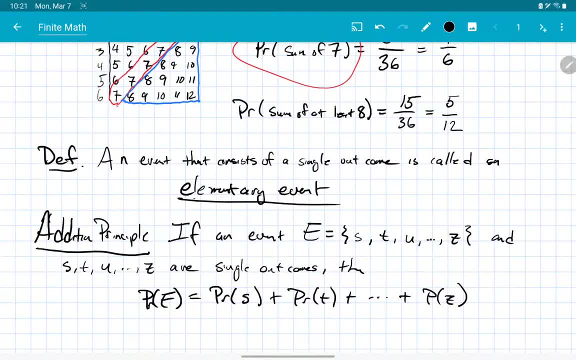 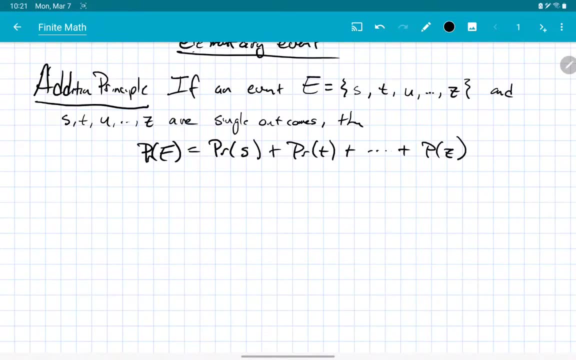 sometimes, however, we will see, events will be hard to write like this, and so we'll need some other way of figuring out how to find the probability. so here's an example we'll do here: considering all three child families, find the probability that the family will have. 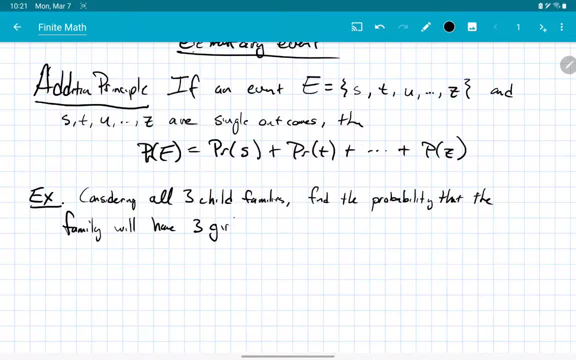 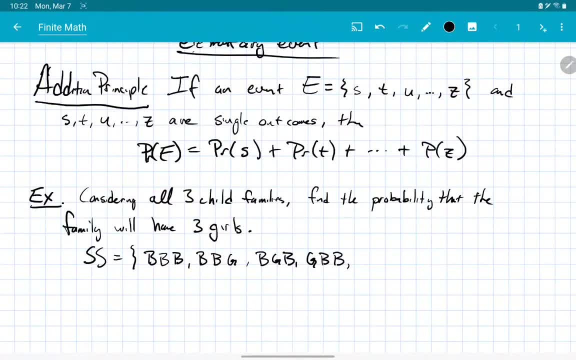 okay, that exhausts the all boy and single girl possibilities. then we have girl girl boy, girl boy, girl boy, girl girl. that exhausts the two girl, one boy possibilities. and then finally, we have girl girl girl, and my pencil doesn't like to work on the far right edge. okay, so we should have eight. 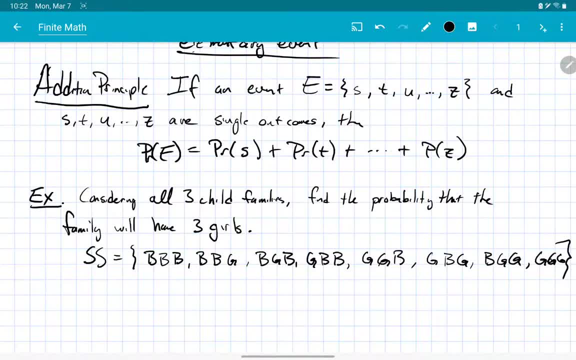 things in this sample space, because two cubed is eight, one, two, three, four, five, six, seven, eight. and how many of these outcomes have three girls? there's only one. so the probability of girl, girl, girl is one eighth, one eighth, twelve and a half percent. so probability of 0.125. 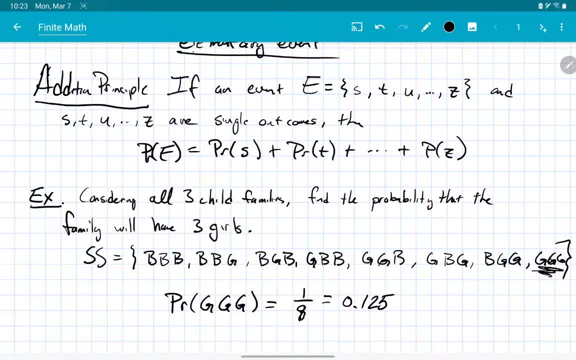 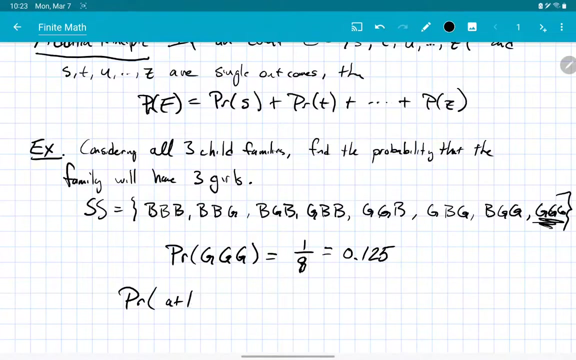 so, given that a family has three children, what is the probability that the family will have three girls? it's 0.125, yes, kayla, so like, so, like. what exactly does it mean to be a single outcome? uh, if i want to say probability of at least two girls, that's not an event, that has a thing, that's. 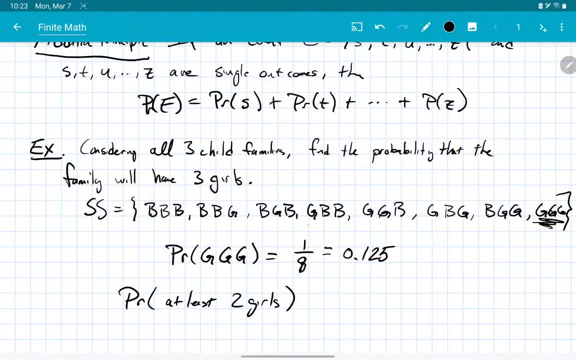 not an elementary event, because there are several outcomes which which lead to that. this outcome, this outcome, this outcome in the last one, yeah, but i can break that into different single outcomes. that's the probability of girl girl boy, girl boy, girl boy, girl girl and girl girl girl, and then the sum of those four probabilities will be what we have here, and so that'll be the sum of those, each of those which has one eighth. so that'd be four eighths or one half. so probability of having at least two girls is one half. 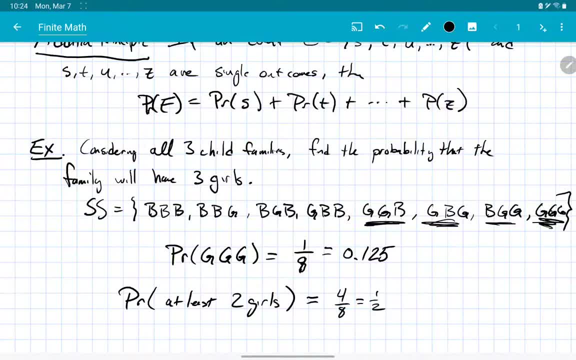 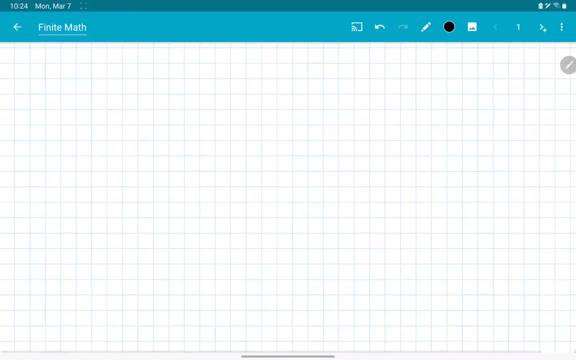 okay now do we have any degenerate gamblers here in the classroom? oh, i'm sorry. responsible gamblers- any responsible? yeah, okay. so odds: you've probably heard of odds, things like three to one odds. so the book wants to talk a little bit about how you go from probability to odds. what, what? 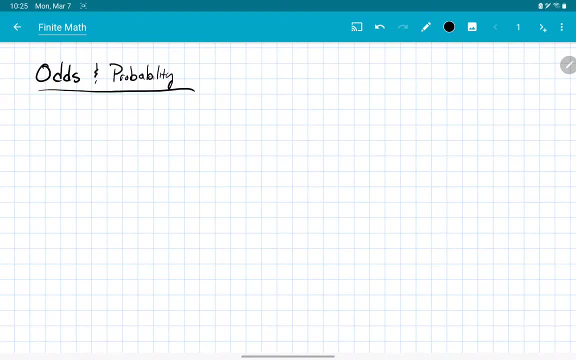 does three to one mean in terms of probability? right, and if you're- if you're- a decent gambler, you probably know this stuff already, right? so three to one odds equals what probability? well, the way you convert a to b odds into probability is a over a plus b. 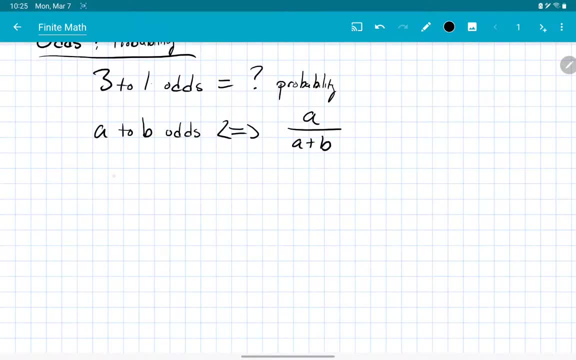 so that means three to one odds converts to: okay, i put the three on the top and then three plus one on the bottom, so this is three quarters or 0.75. so three to one odds is the same thing as 0.75 probability. three to two odds. 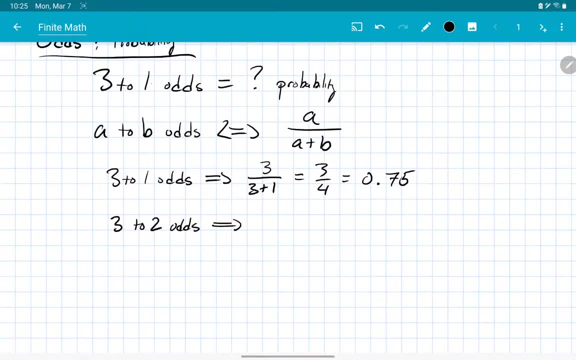 is the same thing as three over three plus two, or three fifths, or 0.60 probability. okay, so three to two odds is not as good as three to one odds, right, okay now. Now the question is how to go the other way, from probability to odds. 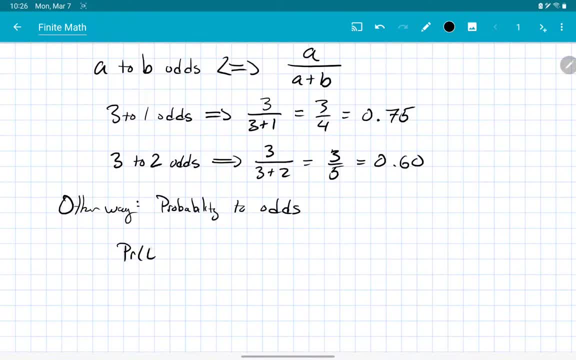 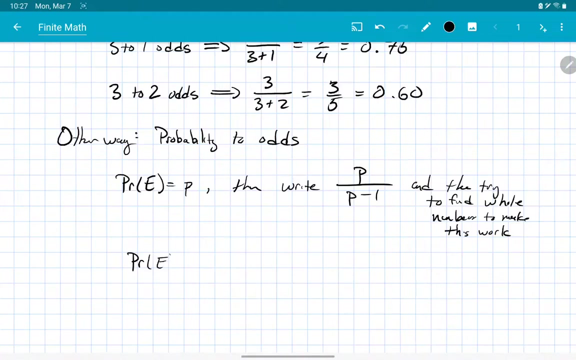 This is a little more difficult. If the probability of an event is equal to p, then you write p over p minus 1, and then try to find whole numbers to make this work. Let's do some examples. Let's do: the probability of an event equals 0.60.. 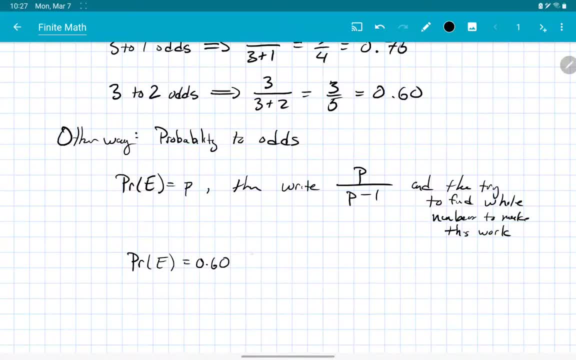 We've seen that already. So if I do what it tells me- p over p minus 1, that's 0.60 divided by 0.60 minus 1.. So this is, of course, 3 fifths divided by 3 fifths minus 1.. 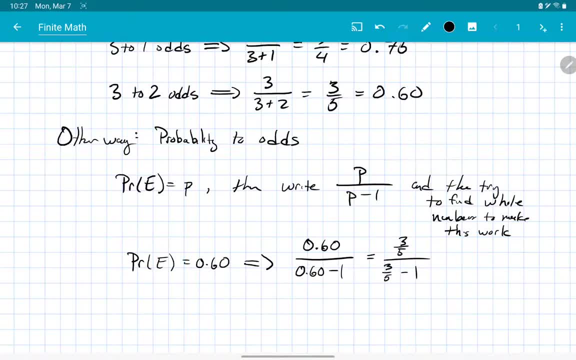 Oh, this should be 1 minus p, not p minus 1.. I'm sorry That doesn't. I've got to erase this. here Makes a lot more sense. One minus p. one minus 3 fifths- Okay. 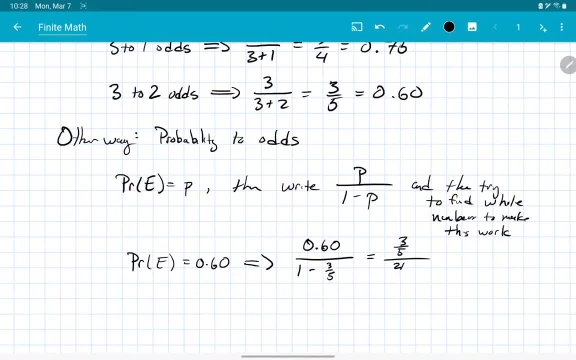 Okay, So it's 2 fifths. So here we get 3 over 2, and that means 3, 2, 2 odds. Okay, The trouble can sometimes be getting this to look like a whole number over a whole number. 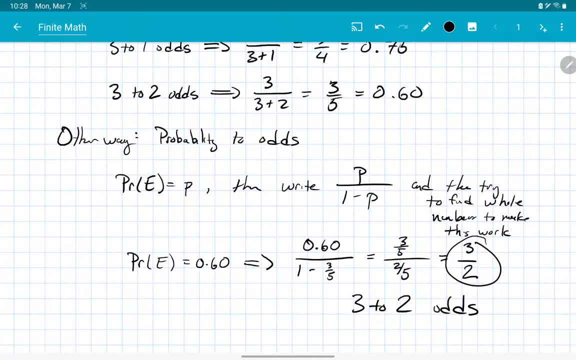 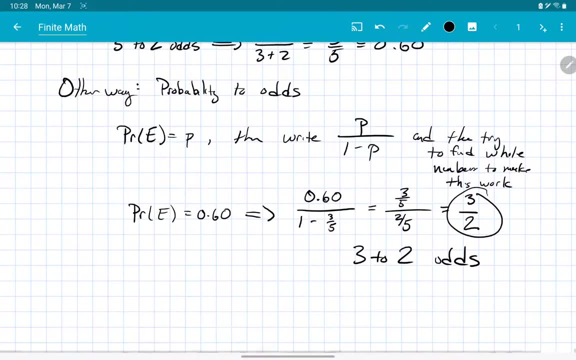 right, You might have to monkey with it a little bit in order to get it as a whole number over a whole number, if it's not a really nice, If it's not a nice fraction already. Another example: The probability of an event. 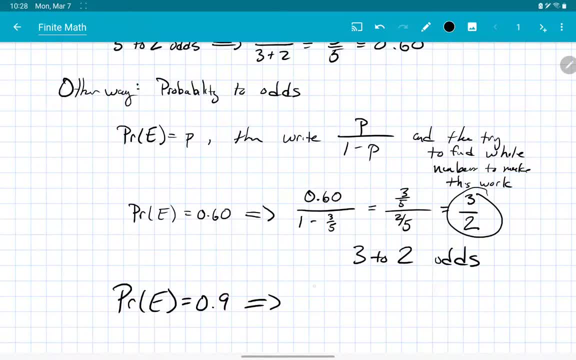 If it's not a really nice fraction already, you might have to monkey with it a little bit. Okay, So the probability of an event is 0.9.. Then we'd have 0.9 divided by 1 minus 0.9.. 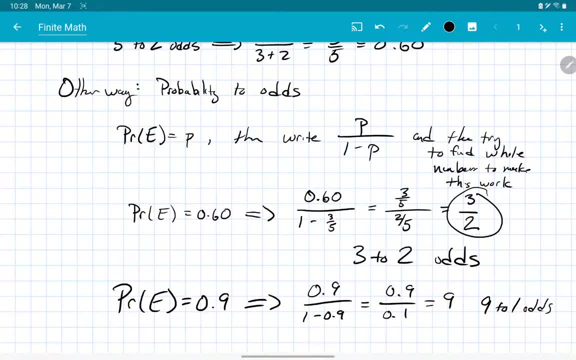 So that's 0.9 over 0.1, which is 9.. So this would be 9 to 1 odds. Like I said, unless you enjoy gambling, this is not that useful Right. I don't know. 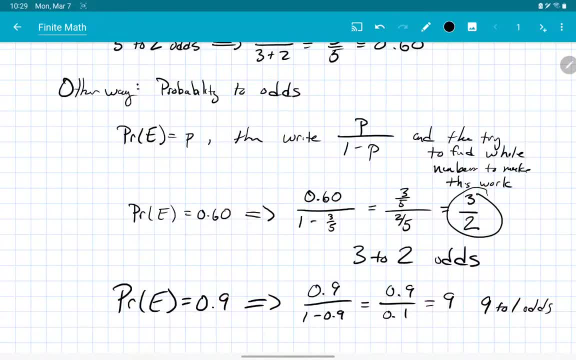 Maybe. Well, you know, if you're going to be in business, you're going to have to think about what you're going to do. What are you going to do? What are you going to do? What are you going to do? 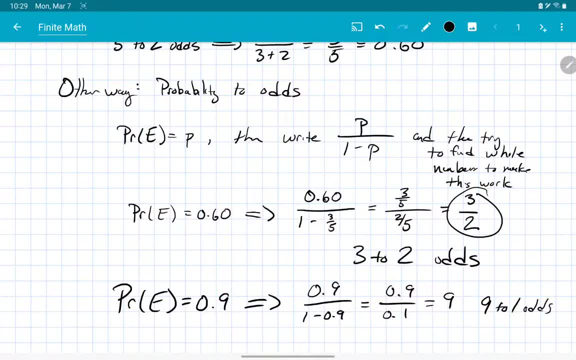 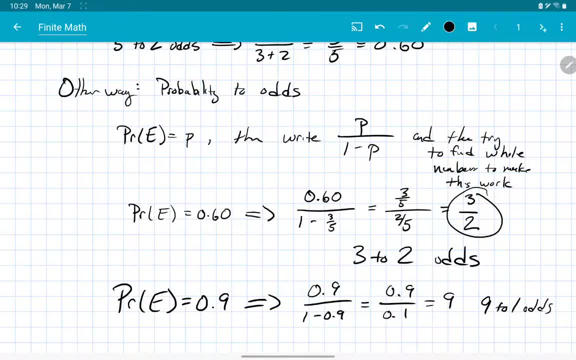 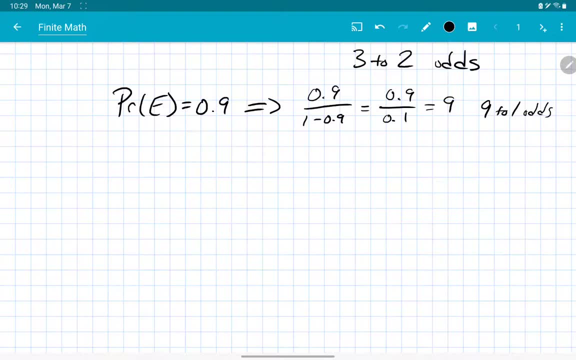 So Seems reasonable. You need to learn something like this, Okay, So let me write down the problems to work on today in class. Make sure you're able to do these sorts of things. Number 17 and Number 21.. And then the homework.